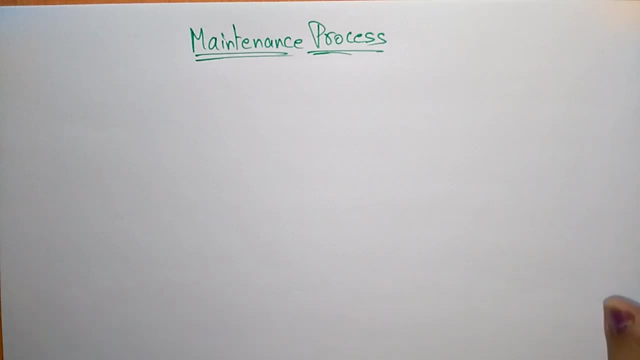 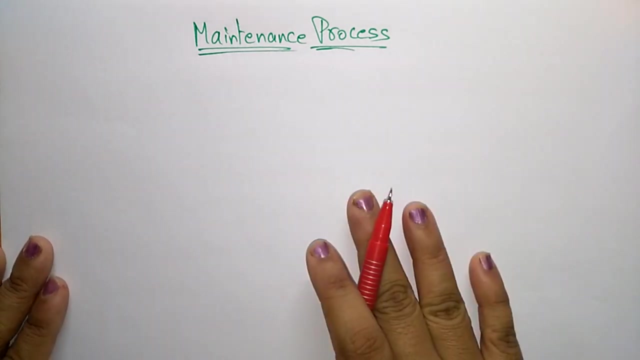 Hi students. coming to the next topic in the software maintenance, that is, the maintenance process. So in the previous video I just given what are the software maintenance and what are the activities- maintenance activities. Now let us see the maintenance process. A maintenance process vary considerably depending on the type of software being maintained. So it's just means based on the different softwares, the maintenance will be varying. Okay, if you want to maintain one type of software, you have to maintain one type of software. So it's just means based on the different softwares, the maintenance will be varying. Okay, if you want to maintain one type of software, you have to maintain one type of software. So it's just means based on the different softwares, the maintenance will be varying. Okay, if you want to maintain one type of software, you have to maintain one type of software. So it's just means based on the different softwares, the maintenance will be varying. Okay, if you want to maintain one type of software, you have to maintain one type of software. 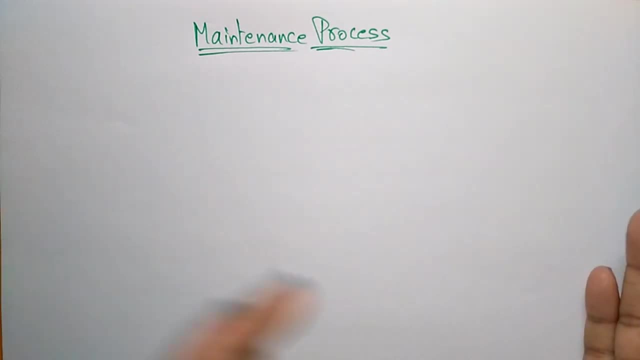 So it's just means, based on the different softwares, the maintenance will be varying. Okay, if you want to maintain one type of software, you have to maintain one type of software. So it's just means, based on the different softwares, the maintenance will be varying. 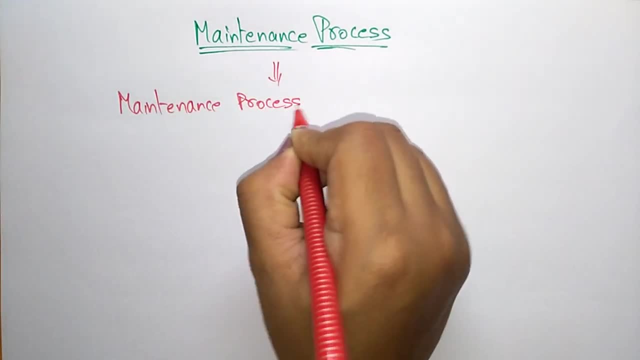 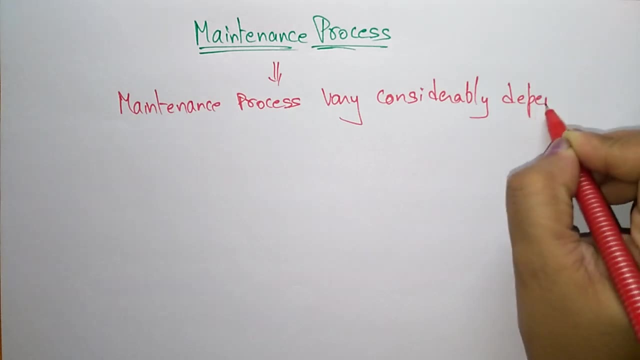 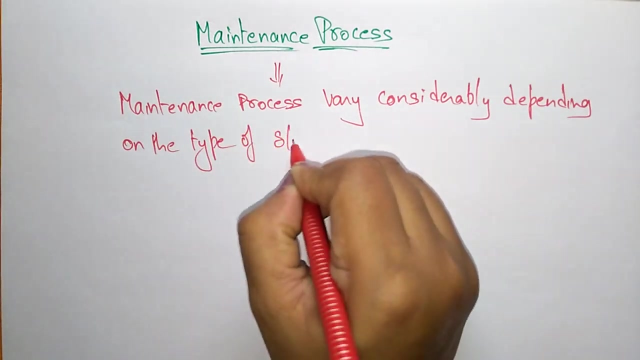 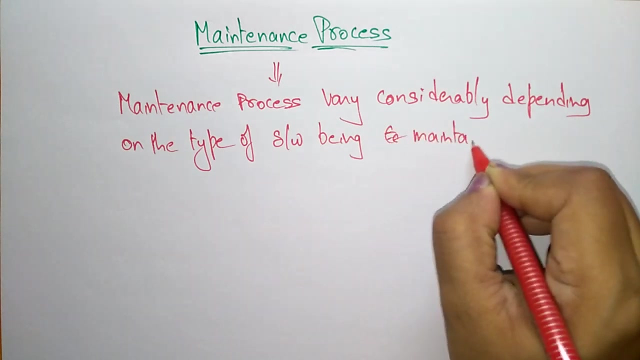 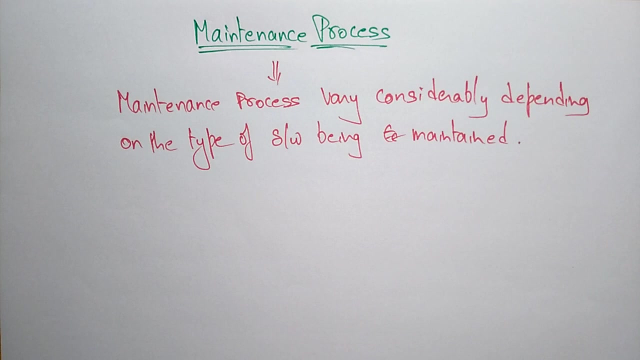 Maintenance process vary considerably, considerably depending on, depending on the type of software, type of software being maintained. So it's based on completely on what type of software you being maintained. So based on that the maintenance process will be work. So actually the most expensive part of software life cycle is a software maintenance process only, okay, the most. 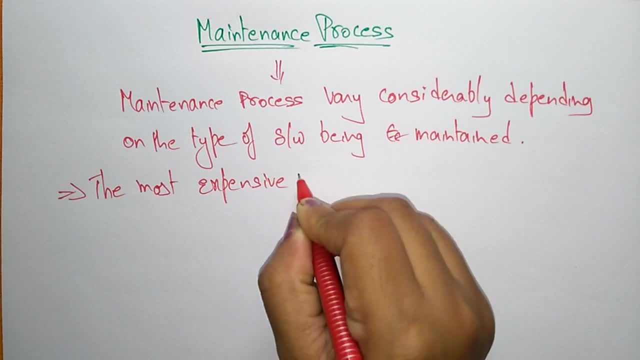 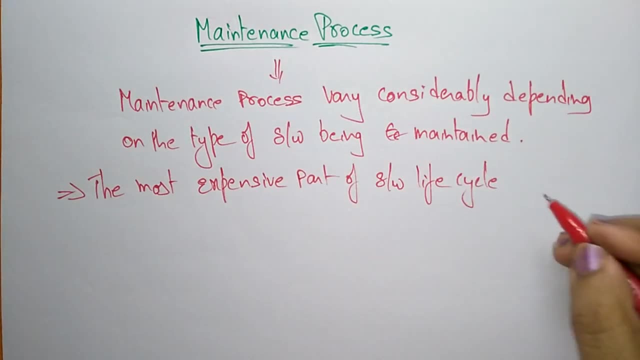 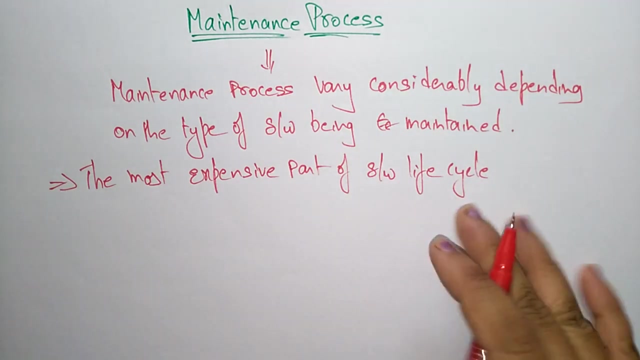 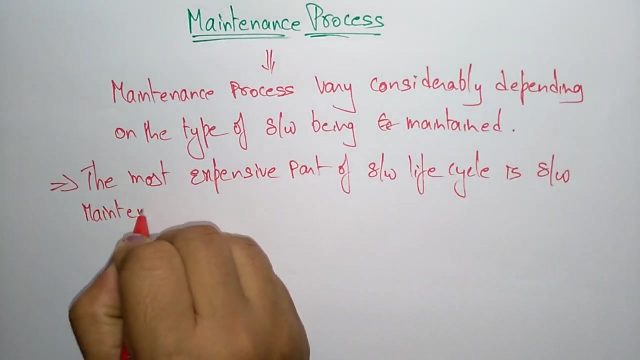 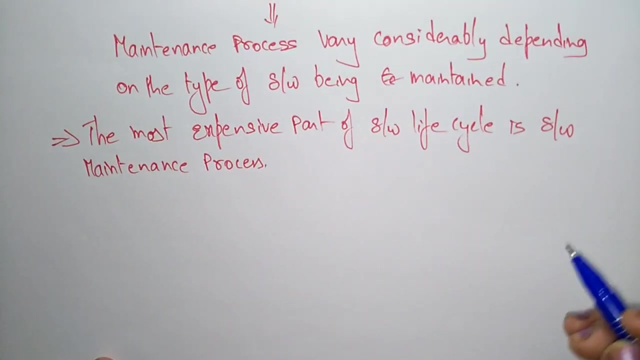 expensive part of software life cycle. if you take any software life cycle from starting of the requirements to the ending of the documentation, means deployment, releasing the product. the most expensive part of software life cycle is software maintenance process and process. now let us see how this uh, a software maintenance process will be. so let 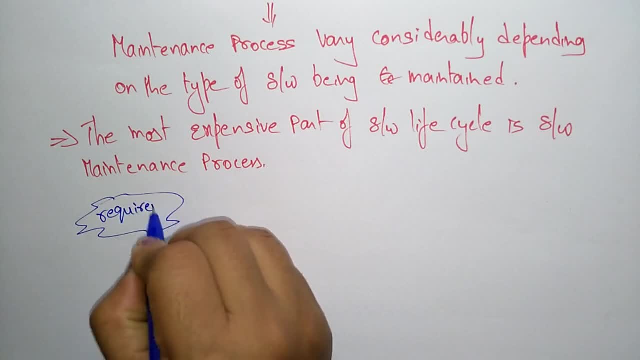 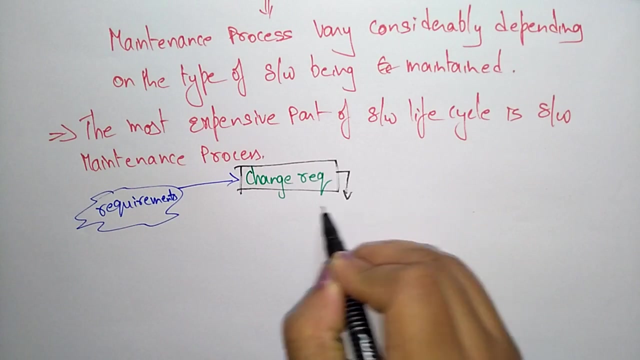 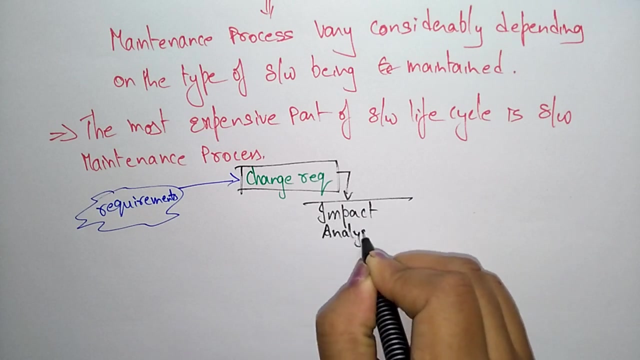 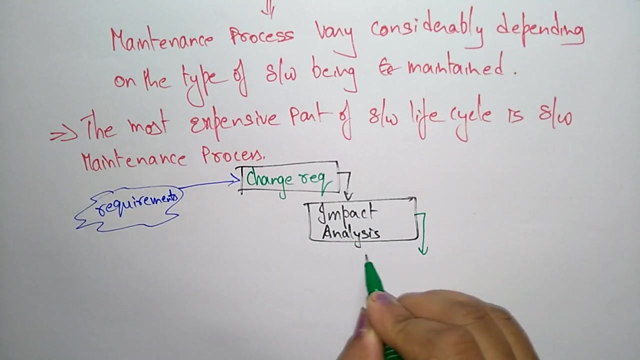 us take the requirements. so these are the requirements. so, from this requirements first is the change request, change requirements. and from after changing the requirements, it impact on analysis, impact, analysis. okay, so again, after that, release planning, release planning. so after release planning, we have to change the design. 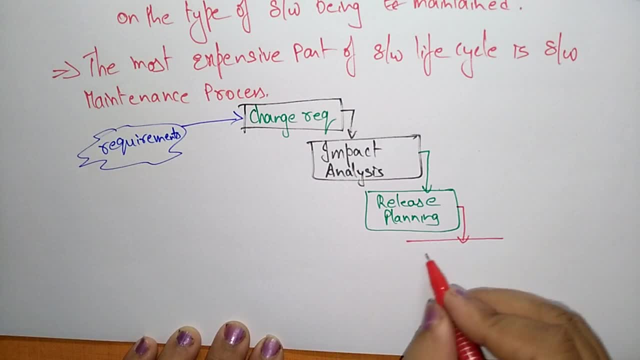 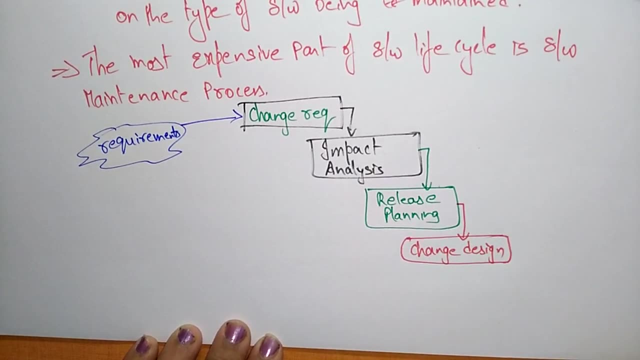 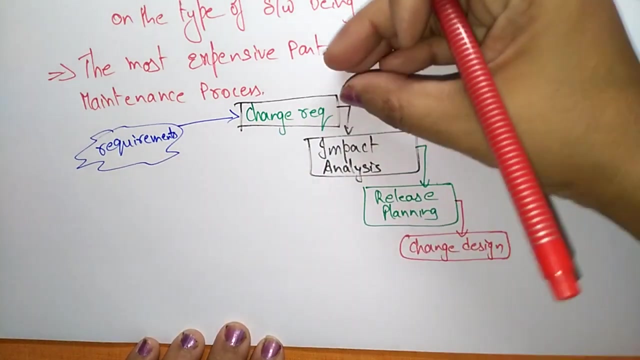 means: uh, so whatever the requirements are changed again you have to change the design. means this is: comes everything after the deployment of the project. means this: the person, the customer, has changed his requirement. suppose any problem is occurred while the system is running, so you have to first change the requirements. means you have to start the work from starting itself. 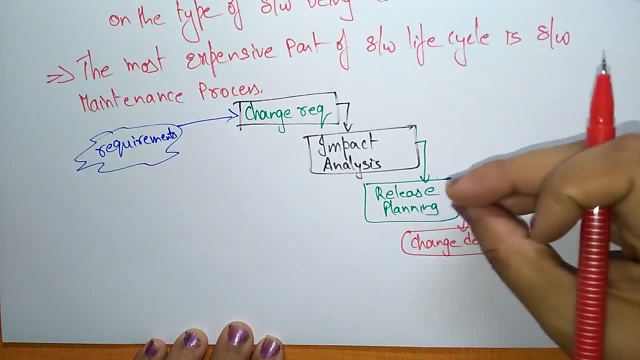 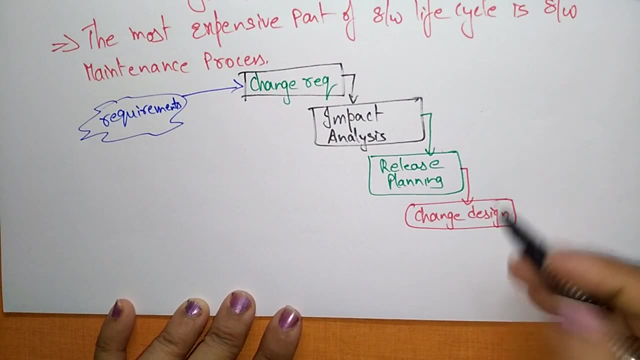 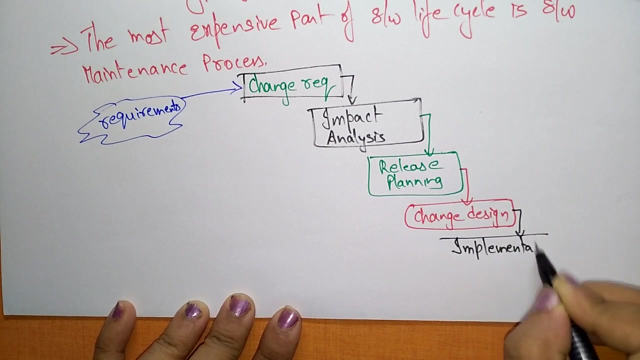 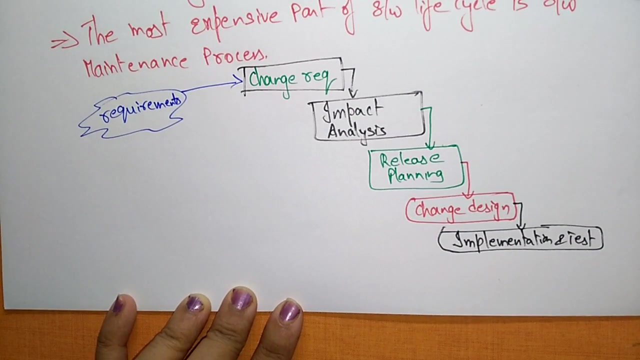 change requirement and it should be on impact analysis and then after that you have to release the planning of whatever the change requirements has taken and then start again the designing. after that change the design, you try to start the implementation work. it's a coding, implementation and test. you have to implement and test and finally you have to 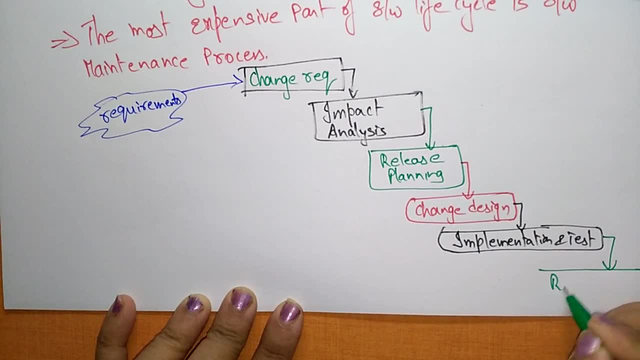 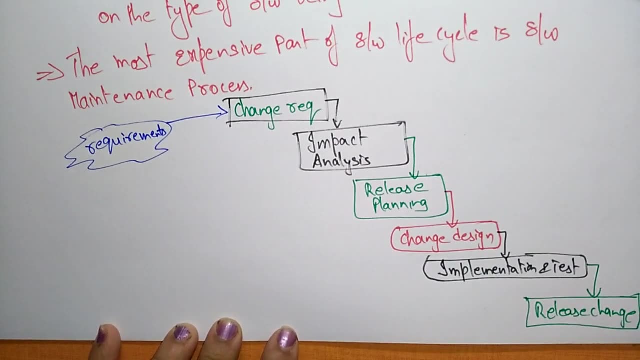 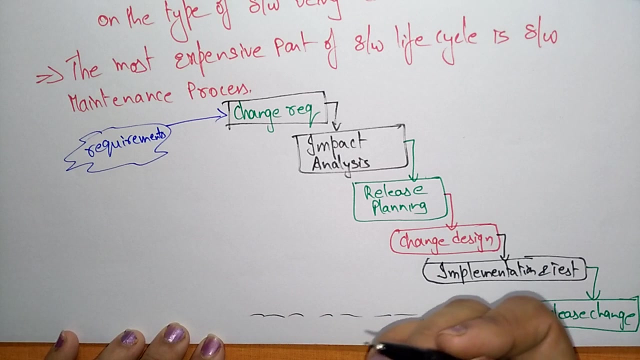 release the changes. so whatever the changes that you have done, that you have to be release changes. so even though you change the system, everything, whatever the customer has asked, still they are having some any doubts means the customer has any doubts, means still a fault is occurring. or he wants to add one more uh point, one more service to the product. 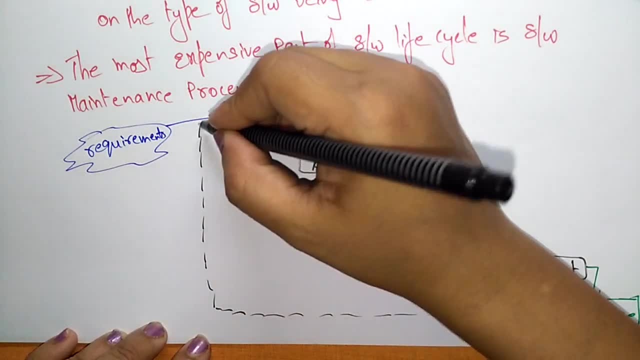 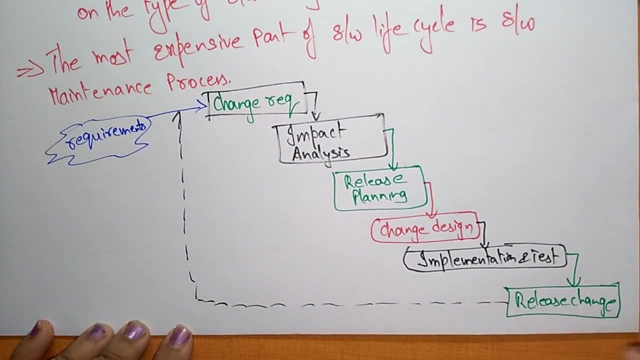 so again, the process will be continued like this. so if it is well and good after the release, change means after the test. if it is well and good the customer will take, otherwise the release has to change again and it has to continue this process. so this is how this maintenance.